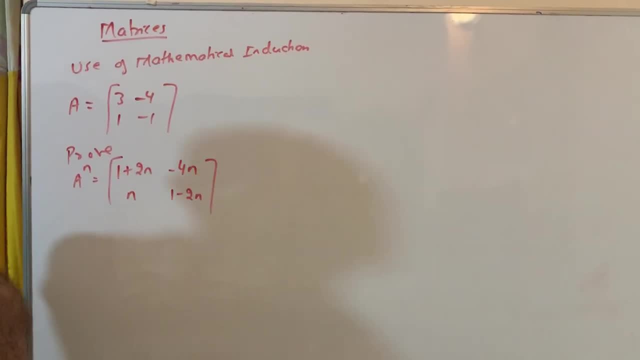 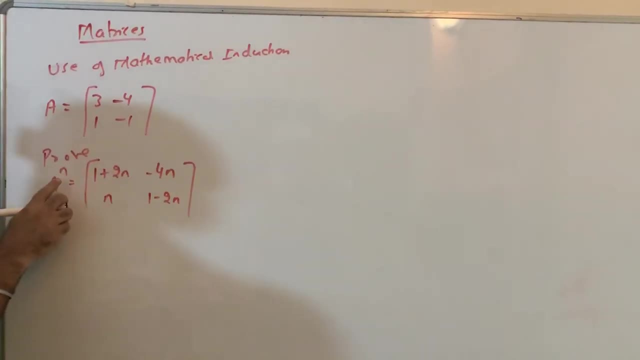 so any doubt is there, send me, but make sure that assignment is done thoroughly. so the last topic is mathematical induction. when you open miscellaneous you will find first, second, third question. so one of that, question a, is this: prove that a, n is equal to this. so you have to use mathematical induction, which you studied in principle of mathematical 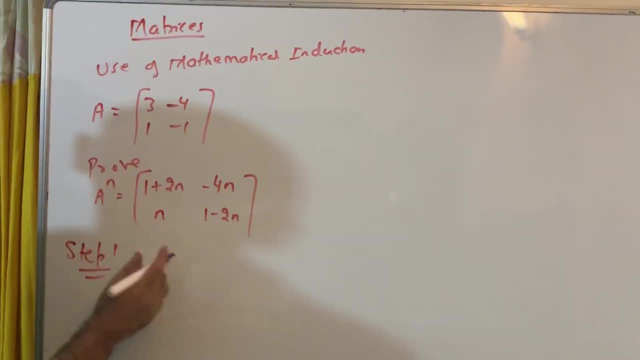 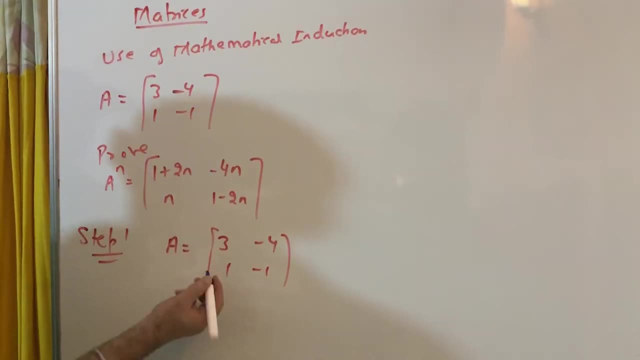 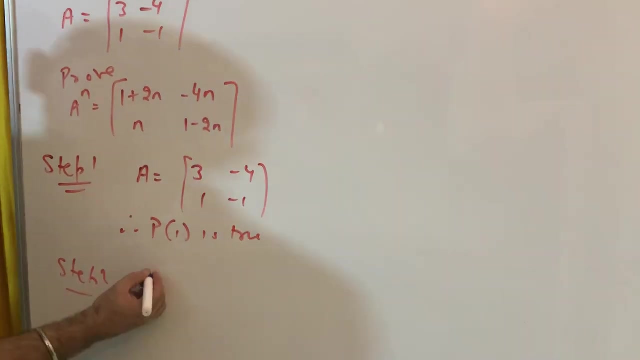 induction which you studied in class 11. so you will put n is equal to 1. so you will put n is equal to 1, you will get: a is equal to 3 minus 4, 1 minus. so that is okay. p of, therefore, p of 1, is what was step 2, if you remember, assume. 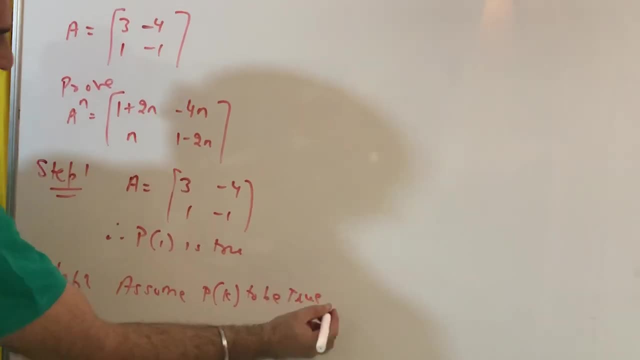 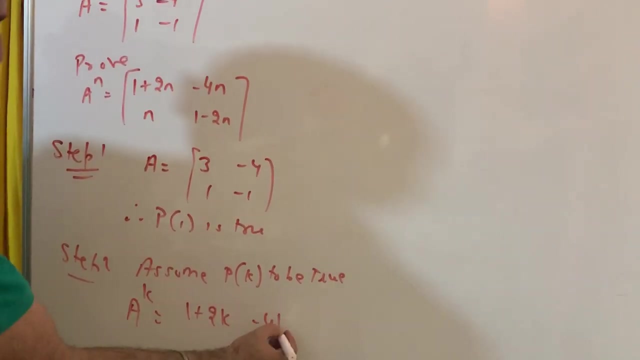 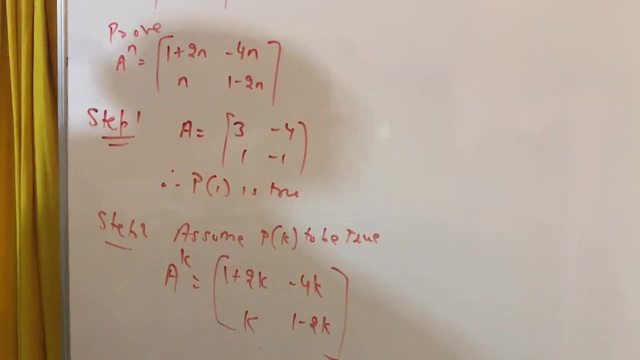 p of k to be true. you will assume p of k to be true. so you will say: a power k is equal to 1 plus 2 k, minus 4 k k and 1 minus 2 k. so you will write like this: so a power k, so assume p of k to be true. 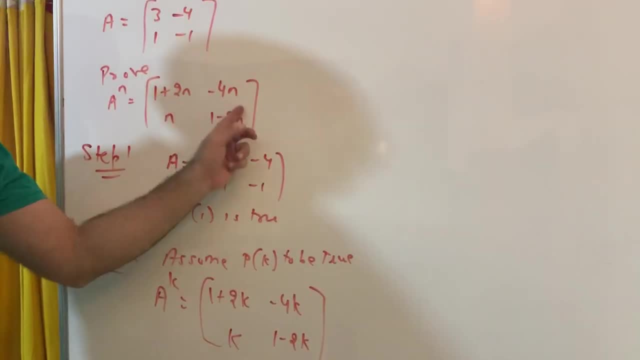 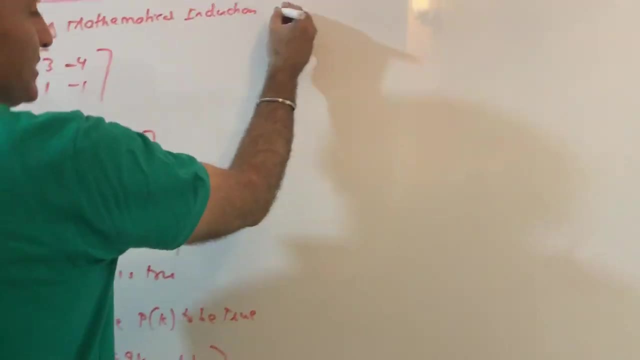 so a power k will be equal to 1 plus 2 k minus 4 k k and 1 minus 2 k. you will write like this: so this you have assumed. now step 3 is so this: let it be 1. so step 3 is what, if you remember to prove, 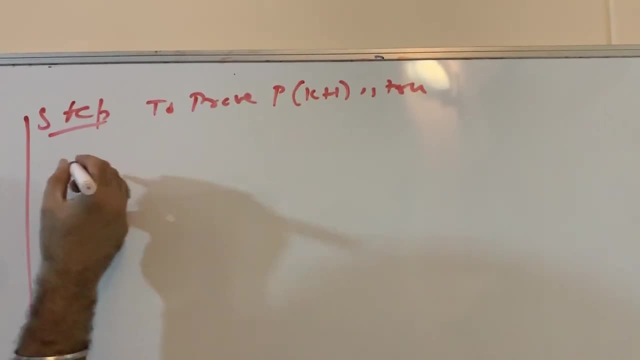 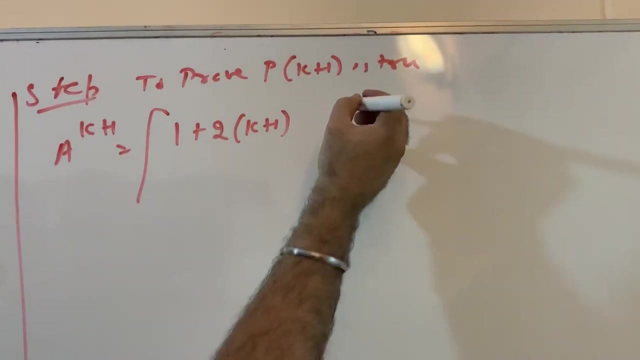 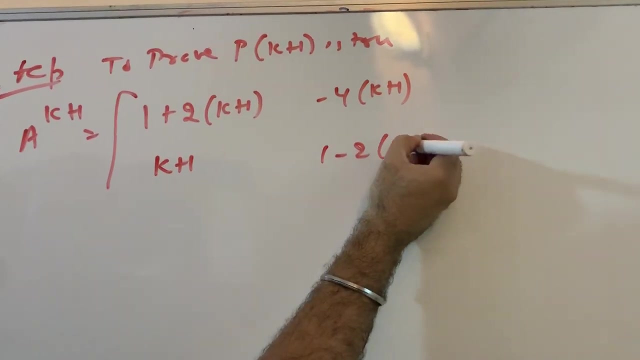 p of k plus 1 is 2. so we have to prove: a k plus 1 is 1 plus 2 k plus 1 minus 4 k plus 1. this is k plus 1. this is 1 minus 2 k plus 1. so this is what we have to. 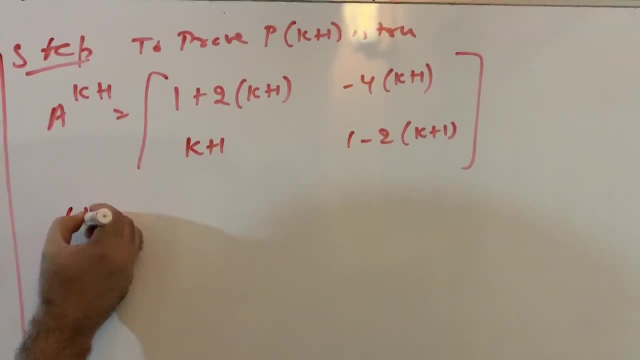 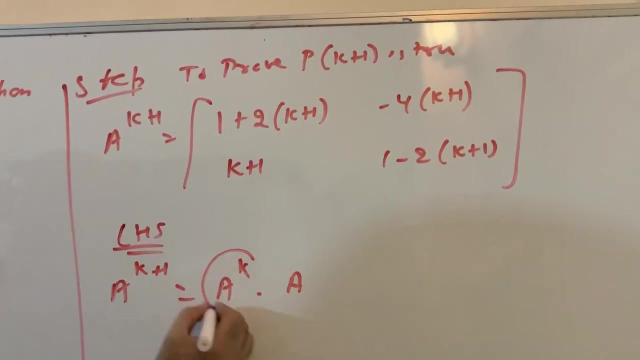 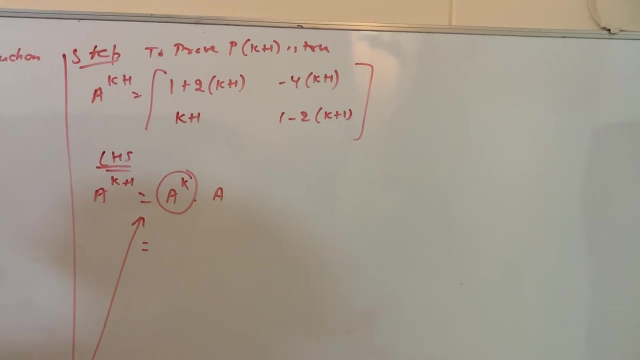 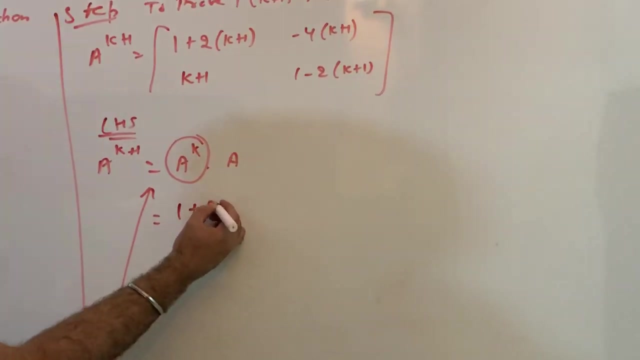 prove. so take lhs, a k plus 1. i can write a k into a. now this a k take from step 2, so this is from this one. so you will write a k. a k will come from here, right, a k will come from here, which you will write it as 1 plus 2 k minus 4 k. 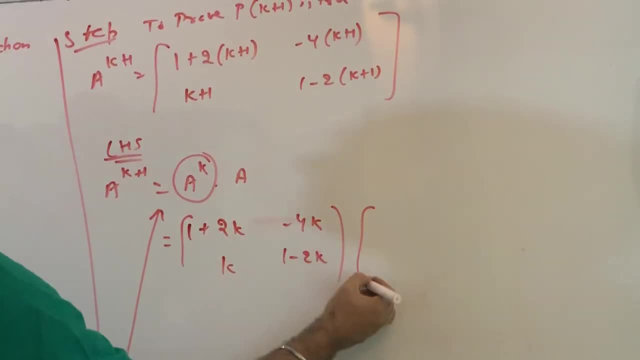 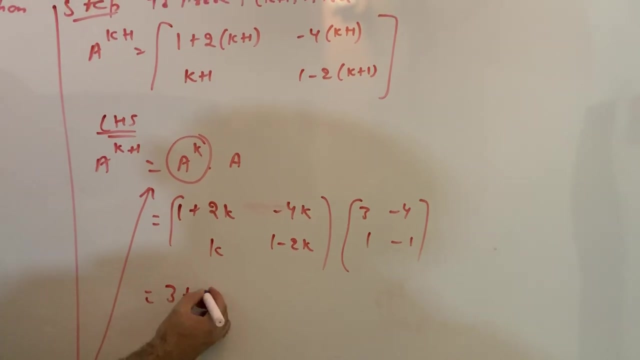 okay, 1 minus 2 k, 1 minus 2 k, 1 minus 2 k, 1 minus 2k And a, you know, is 3 minus 4,, 1 minus 1.. So just multiply now, So 3 plus 6k minus 4k, right? 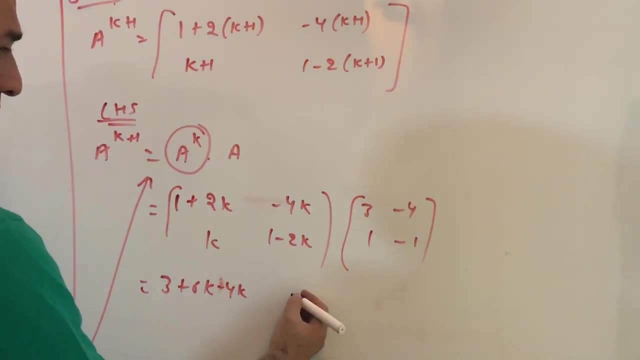 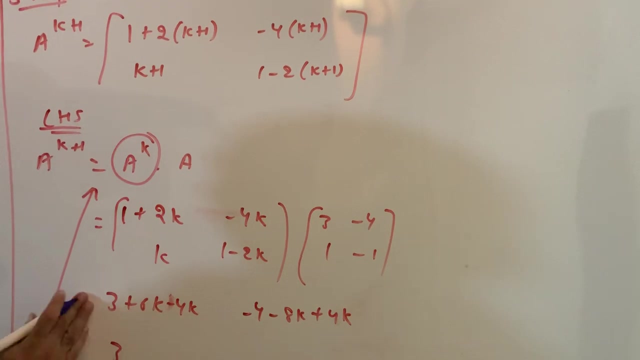 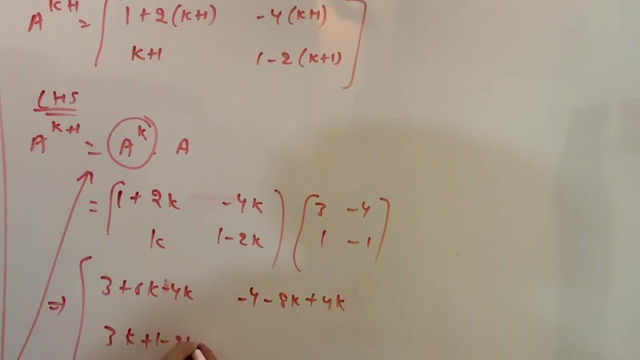 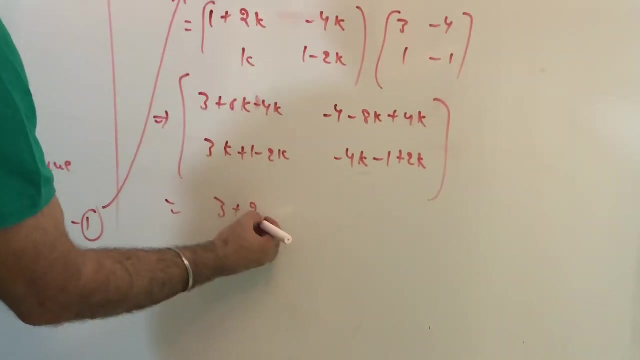 This: you can write minus 4 minus 8k plus 4k. So this you can write: 3k plus 1 minus 2k, minus 4k minus 1 plus 2k. You can write like this: So this will become 3 plus 2k. 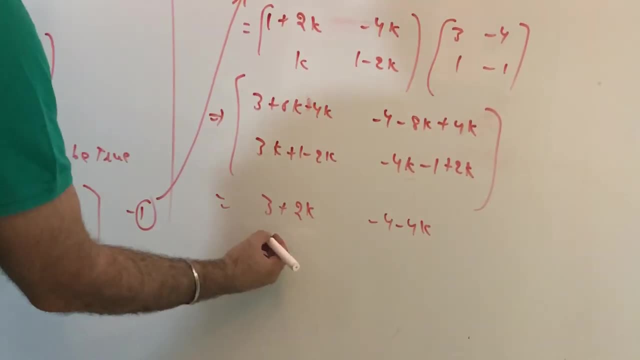 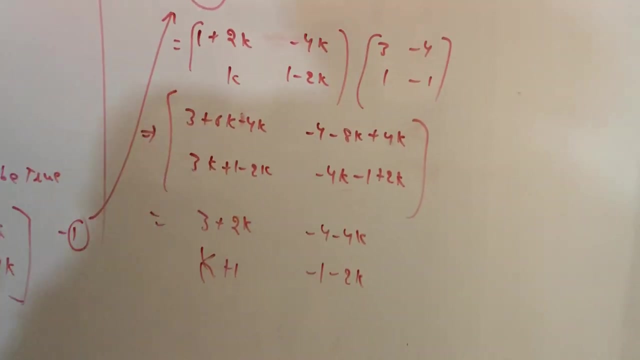 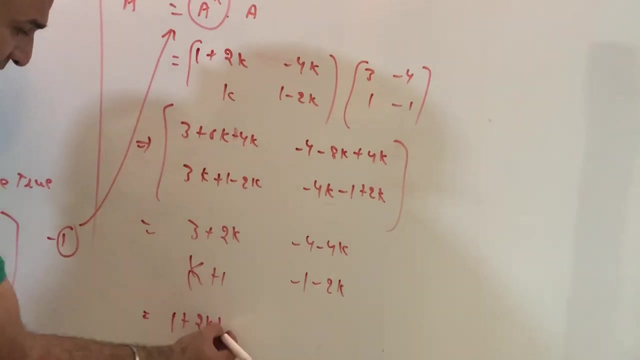 This will become minus 4 minus 4k, k plus 1.. This will become minus 1 minus 2k. So this. So this I can write. if you see 1 plus 2k, I will write it here. 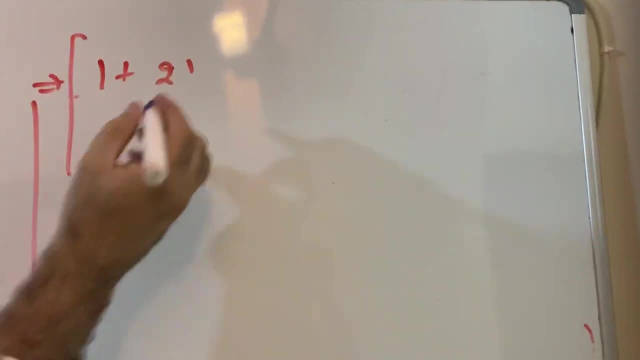 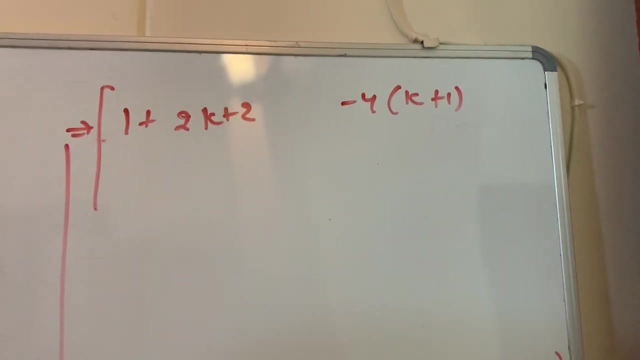 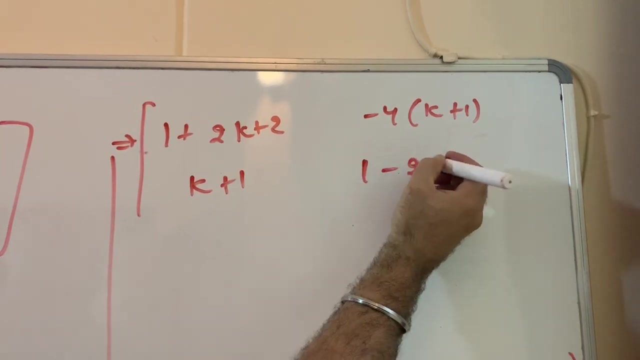 1 plus 2k plus 2.. 3 plus 2k: This I can take minus 4 common k plus 1. This is already k plus 1 form. This I can write minus 1.. I can write 1 minus 2 minus 2k. 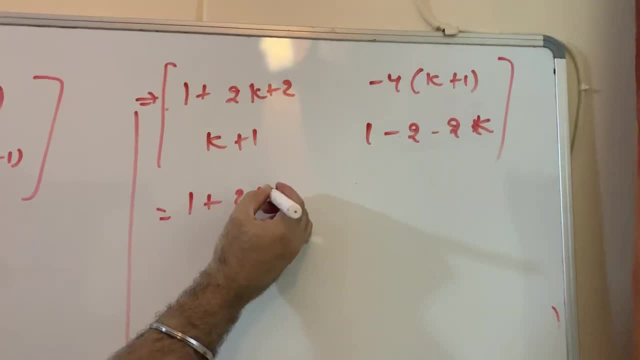 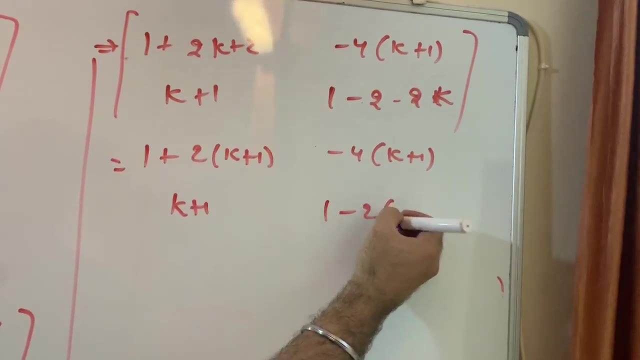 So I can write like this: So I can write 1 plus 2k plus 1 minus 4k plus 1k plus 1 and 1 minus 2k plus 1.. So this is equal to p of k plus 1, or is equal to i hs. 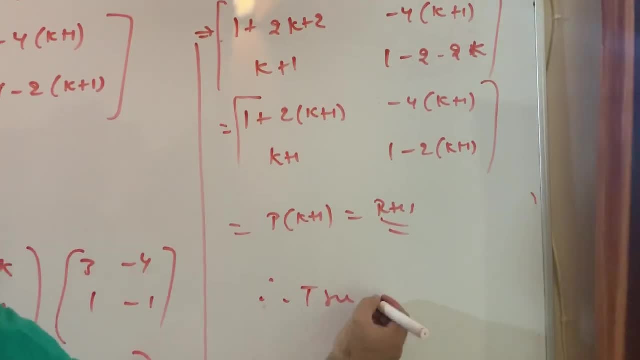 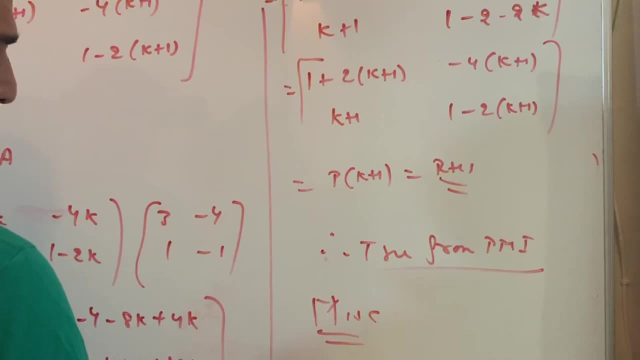 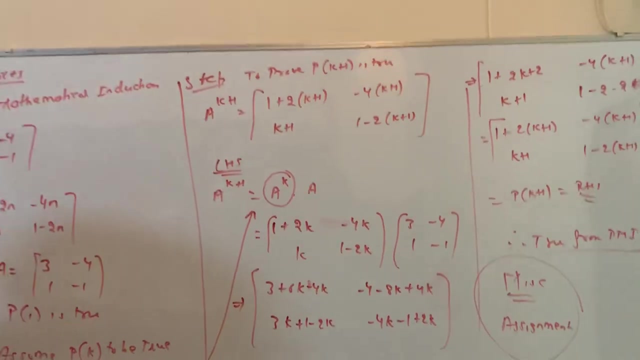 That is what you have, So you can write for from. So please go through this, Solve miscellaneous assignment, Assignment And very soon you will have test And next class. I will start with determinants, Thank you. Any doubt is there, tell me. 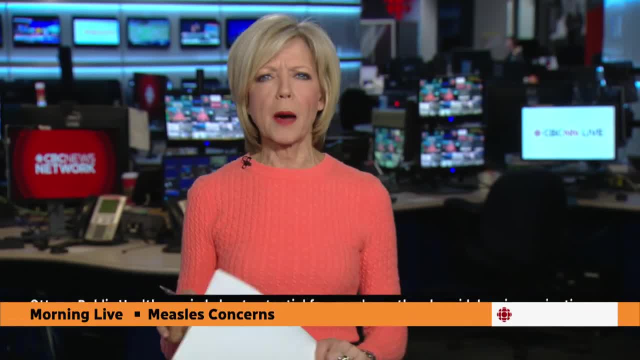 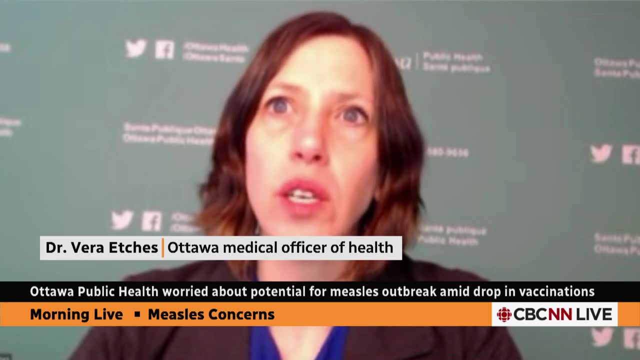 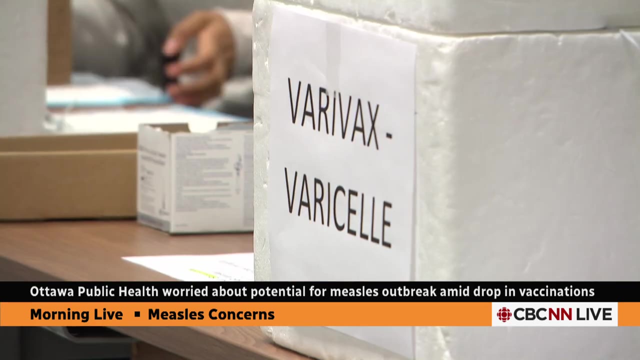 Officials in Ottawa are taking action to try to stop a potential outbreak of measles. The re-emergence of certain vaccine preventable diseases is being seen across the world and it is cause for concern. Officials with Ottawa's public health raised concerns. They had a meeting of the health board.